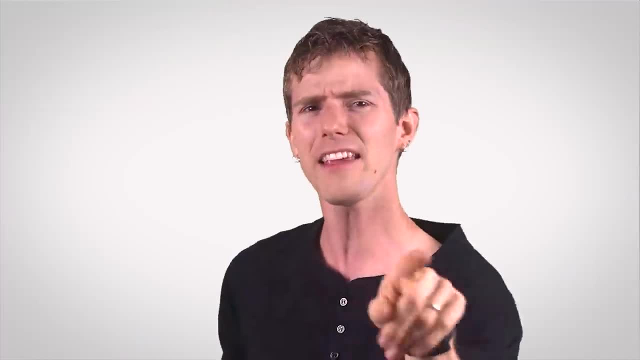 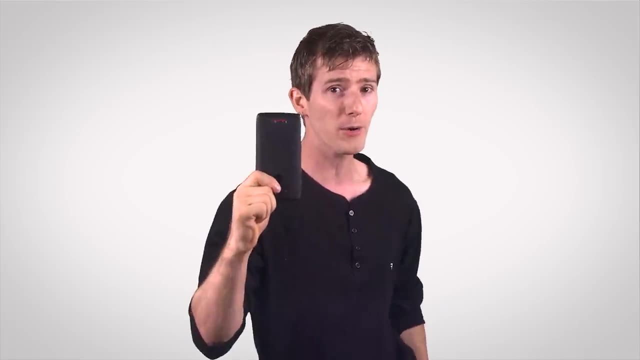 Don't these things need some sort of operating system too? Yes, they do, and they actually differ from PC OS's in a few key ways. We'll start with the ones designed for battery-powered devices like phones and tablets. These might seem like they should be very different from a desktop OS. 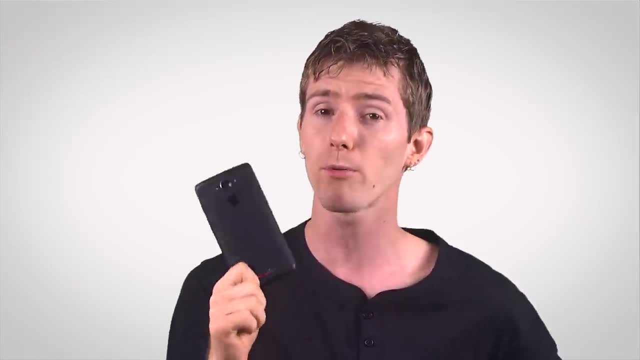 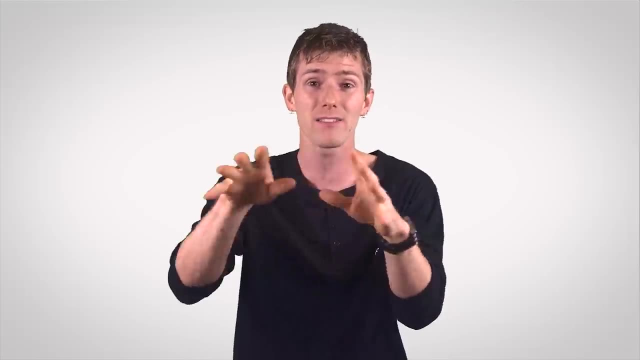 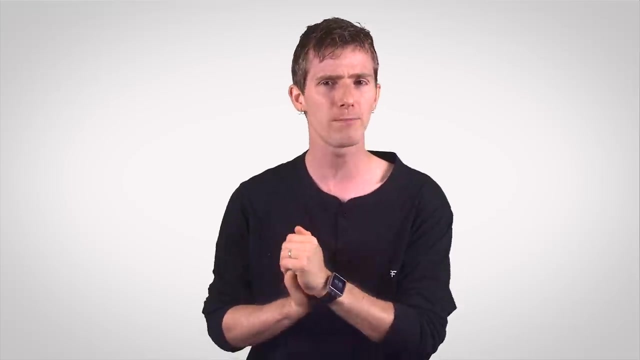 but thanks to the incredible performance of modern mobile processors, top mobile OS's, including iOS and Android, are multi-tasking operating systems capable of balancing multiple background tasks and user input with grace and poise. usually, But it hasn't always- been this way. 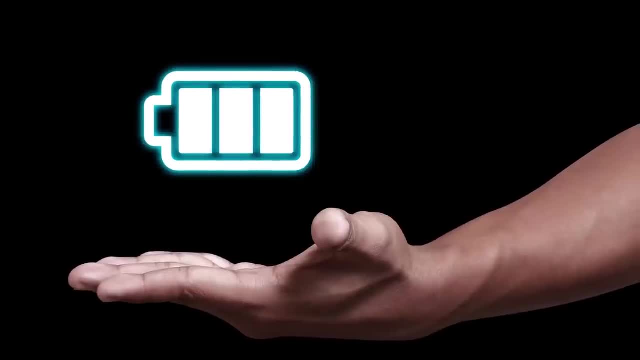 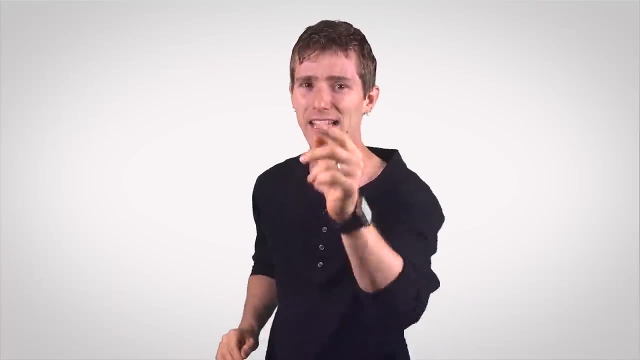 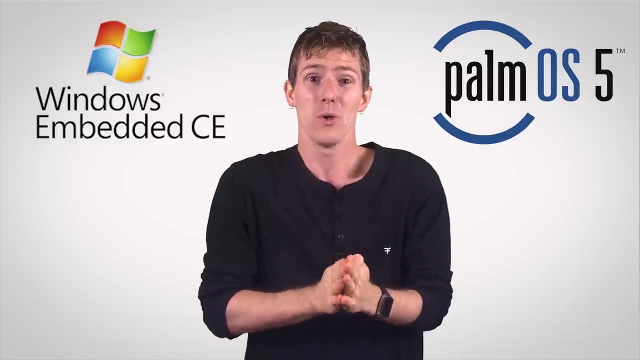 In the early days of mobile computing, battery life and performance were much less plentiful than they are today, so the embedded operating systems were king, examples of which being Windows, C, VE and Palm OS. They had limited functionality and could only handle one task at a time. 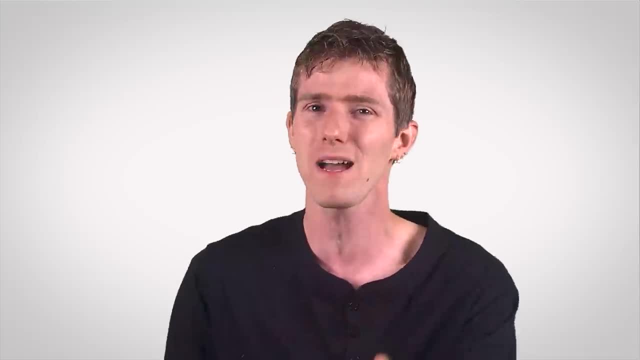 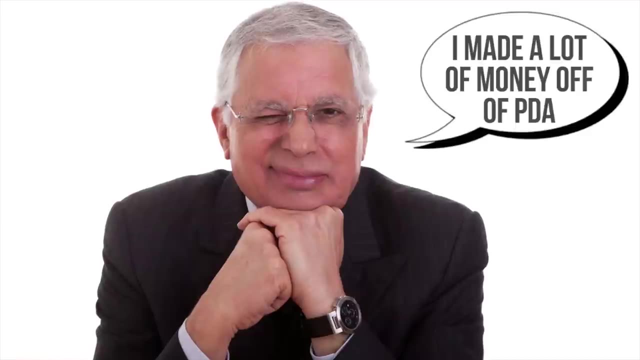 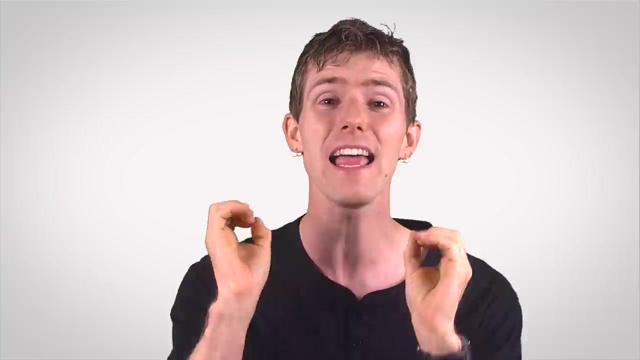 so by today's standards they'd be considered pretty useless on a phone, but my grandpappy tells me they were essential for these strange devices called PDAs. But seriously, even though the days of pocket PCs are behind us, embedded OS's are still essential for many other low-powered, limited functionality devices. 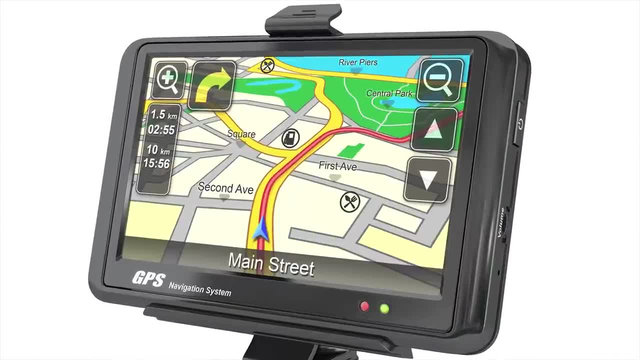 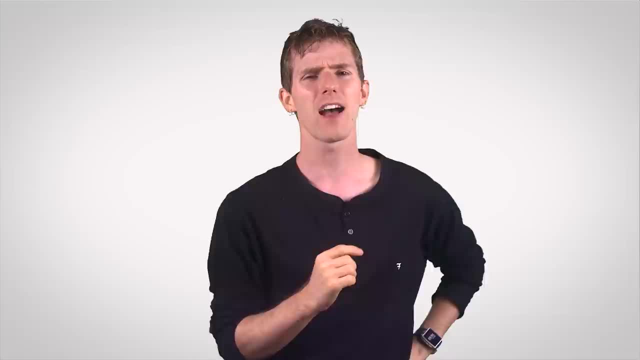 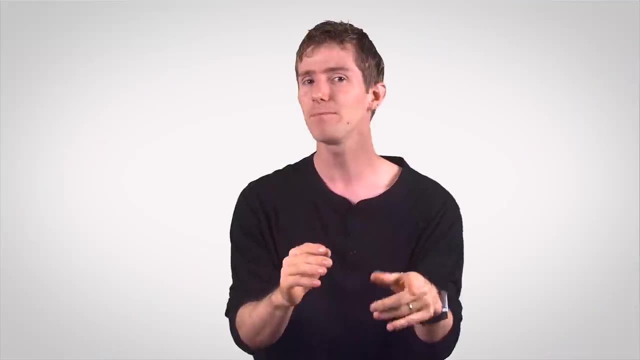 like media players, video cameras, GPS units, fancy dishwashers or even the networking router, which is currently allowing you to enjoy this video. At certain times, though, such as when dealing with heavy machinery, a system's need to process requests quickly and reliably. 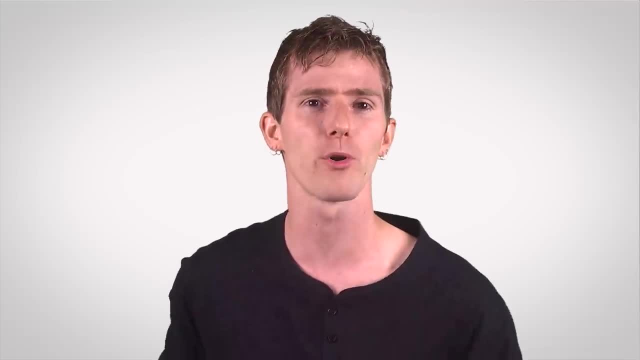 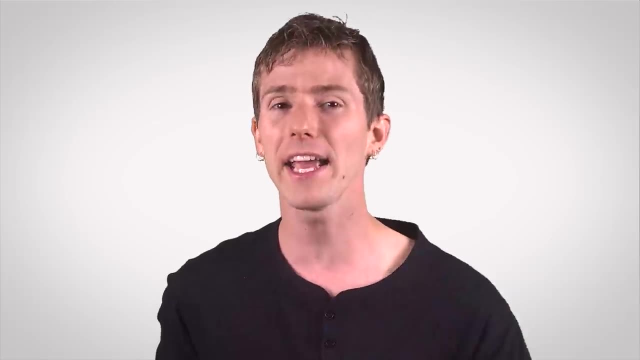 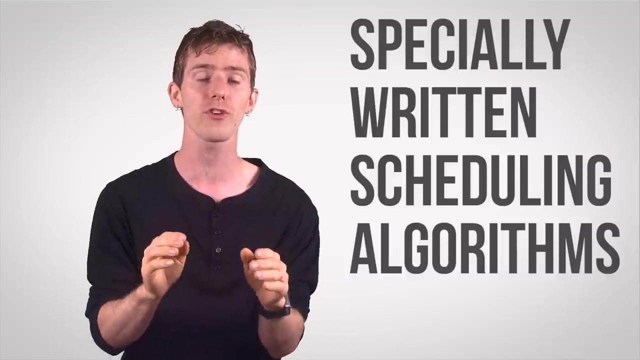 will trump its need to be flexible and easy to program for. In these instances, programmers turn to real-time operating systems, a special variety of embedded OS which, like their name suggests, use specially written scheduling algorithms to ensure that vital information is processed in designated orders. 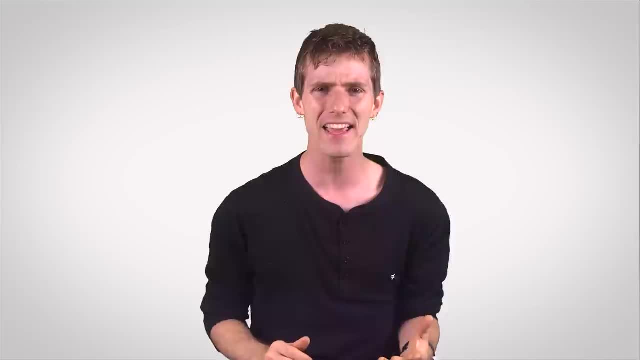 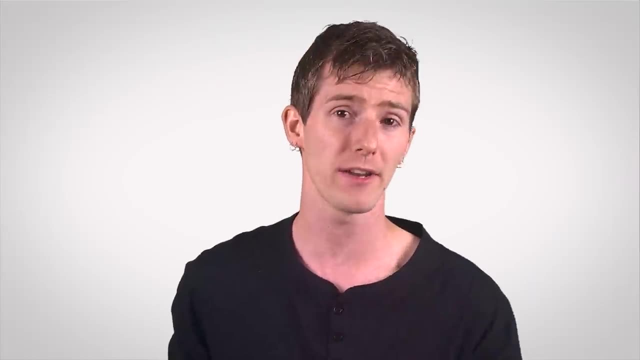 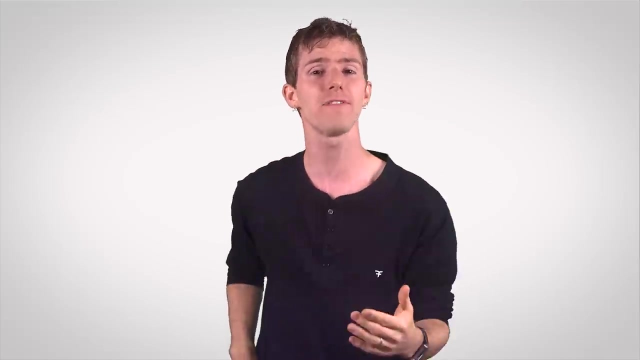 and within specified time windows, instead of dynamically switching between processes based on resource availability. They're very similar to other embedded OS's in that they are often developed in tandem with a dedicated piece of hardware intended to run them, and they can be found on shipping stations. 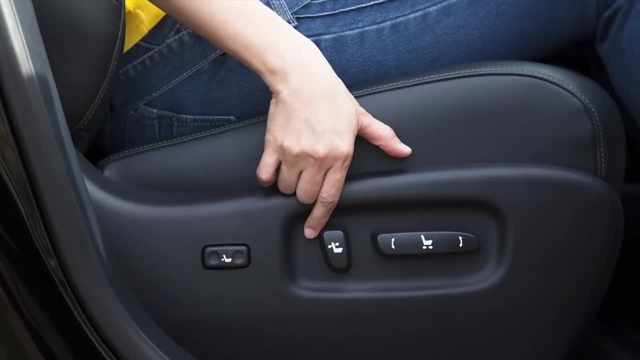 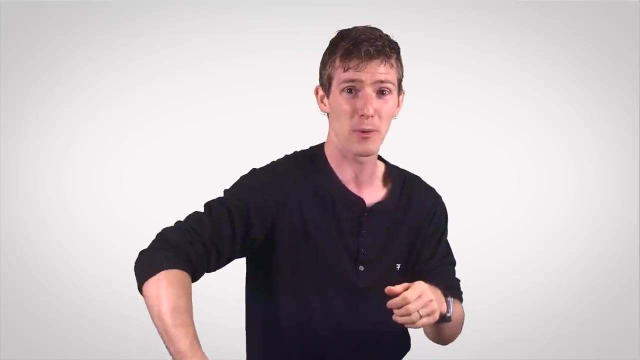 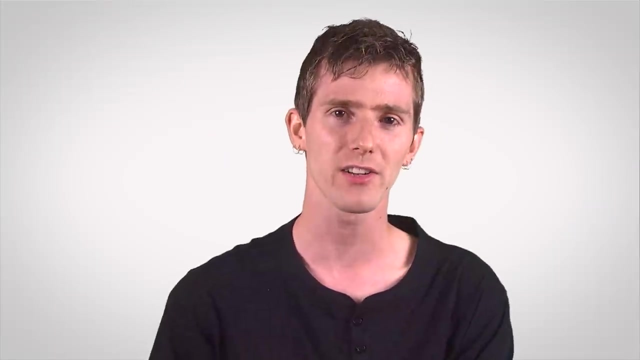 robotic assemblies, assembly lines and medical equipment in our vehicles, and they're very useful for ensuring that our automatic emergency brake doesn't get stuck behind our seat. warmer activation in an OS processing queue as we careen directly towards a brick wall, Switching gears entirely. there's another car thing for ya. there are operating systems that try to avoid normal hardware constraints by utilizing network connections to run virtual OS's, like servers, which can operate several systems simultaneously, or systems that pool resources between even many more machines at a time. 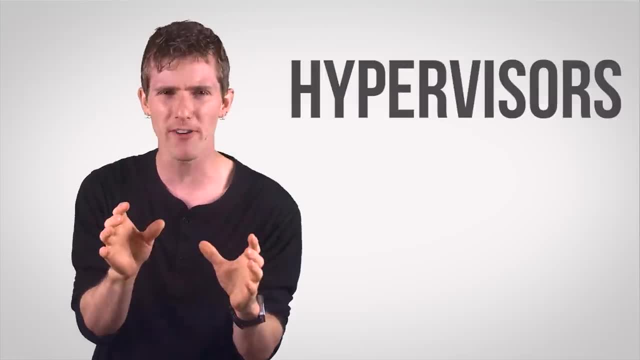 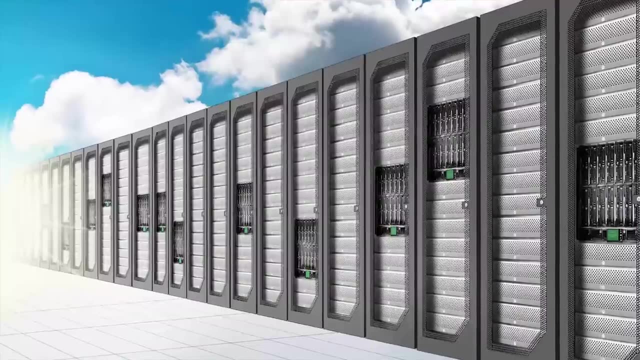 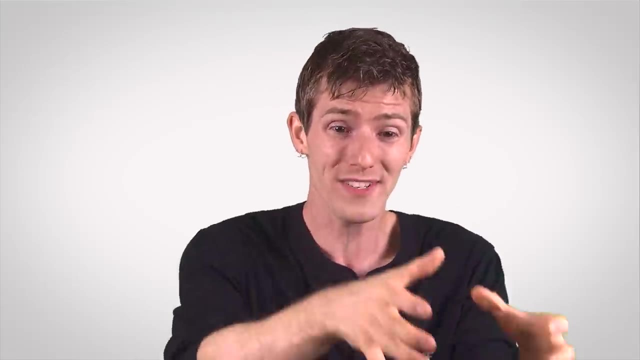 The first style. templated systems use hypervisors to create several virtual machine images on one extremely high-powered system, which users can then access via a network. These machines appear from the outside to be their own dedicated pieces of hardware, but they're not. 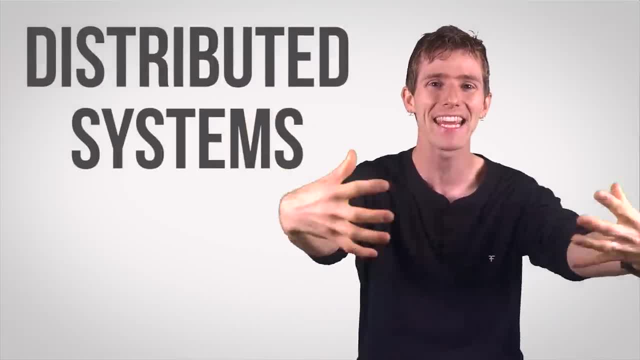 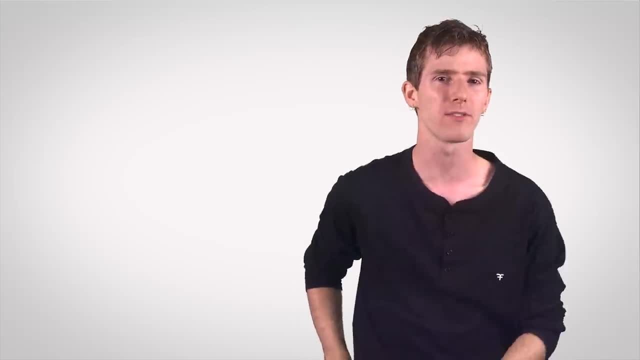 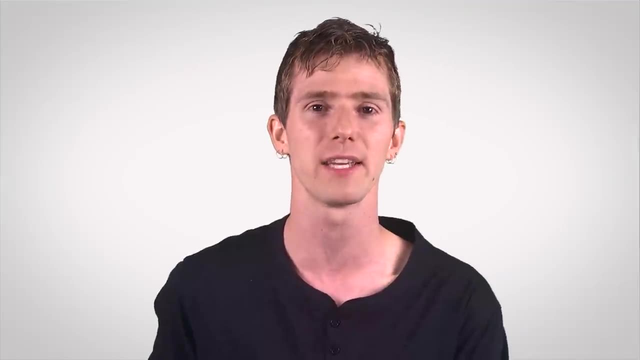 And a second style: distributed systems combine and then allocate the resources of many physical machines, even over the internet, to solve problems like calculating protein folding to help fight diseases. Uh, shameless plug for the Linus Tech Tips folding team, by the way. 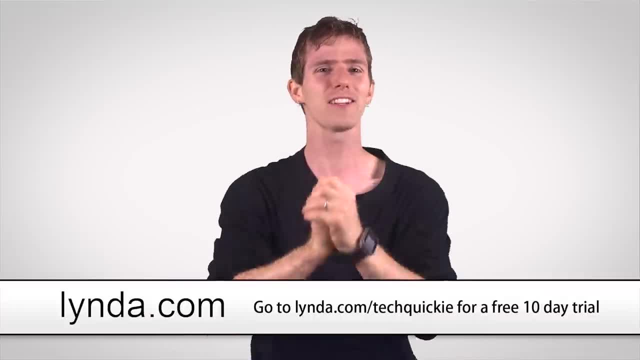 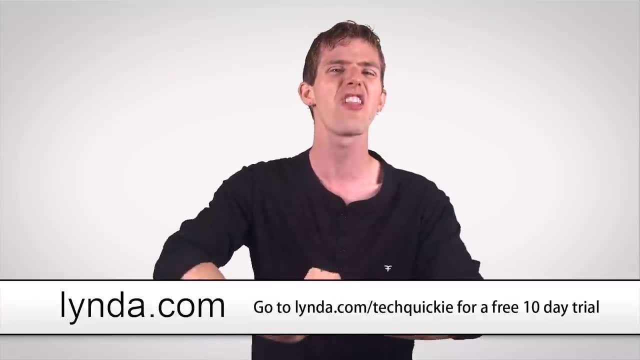 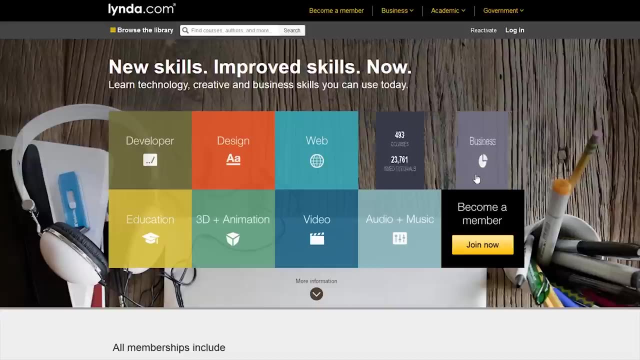 Speaking of shameless plugs: Lyndacom. Lyndacom allows you to watch and learn from top experts who are passionate about teaching. They have thousands of video courses that you can stream on demand and learn on your own schedule, and you can browse each course transcript to follow along. 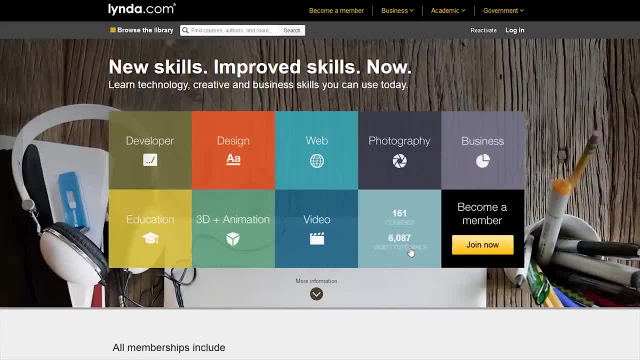 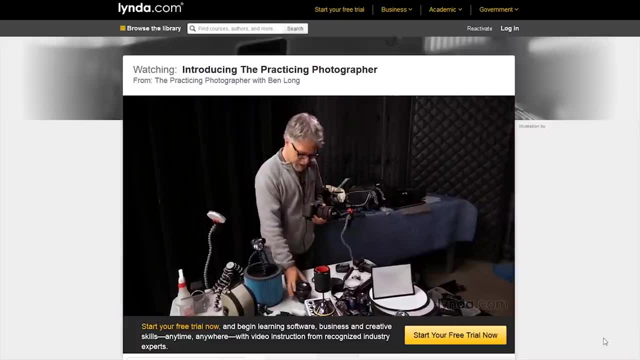 or search for an answer and skip to that point in the video. You can take notes as you go, You can download tutorials and watch them on the go, including access on your iOS and Android device, and you can create and save playlists of courses you want to watch. 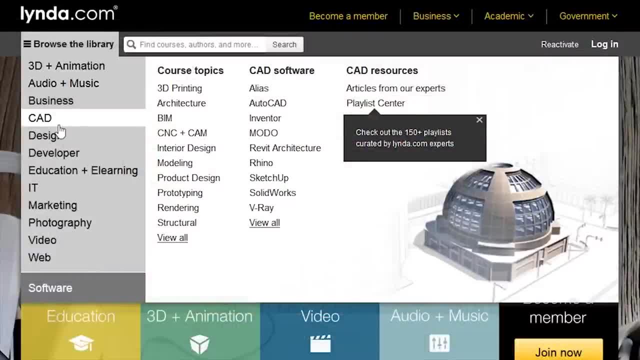 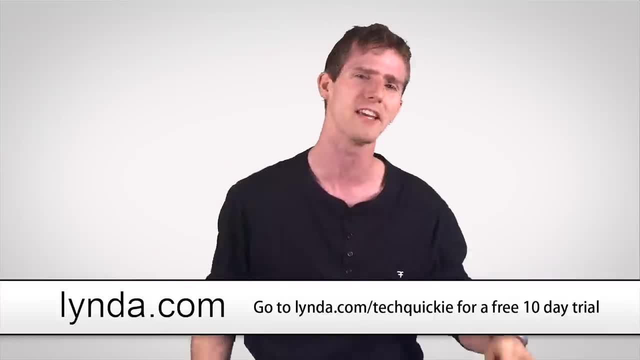 to customize your learning path or share with friends, colleagues and team members. So what could you learn? Well, I don't know. It's not in my notes for today, but it's okay, I've done enough of these Lynda spots to have a pretty good idea. 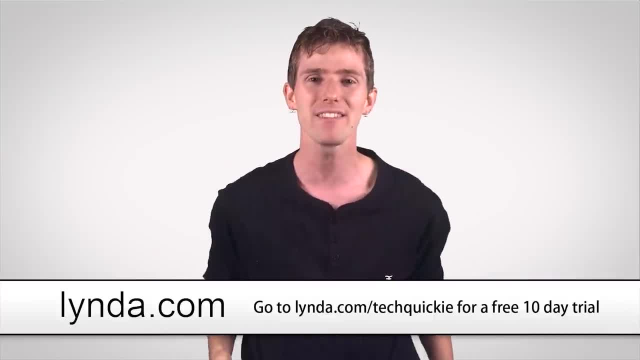 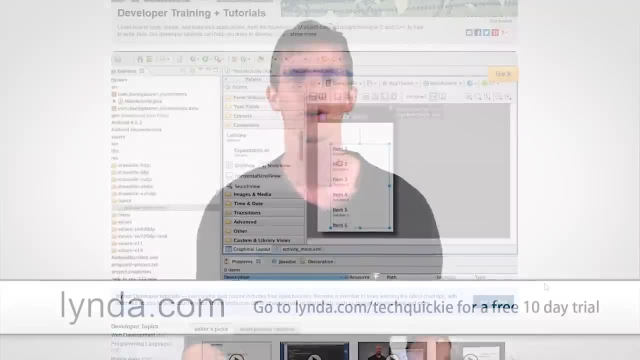 Things like digital photography, video editing, business, key applications that you're going to need if you want to like, get a new job in the digital age, like Microsoft Word, Office- and well, Word is part of Office, whatever. 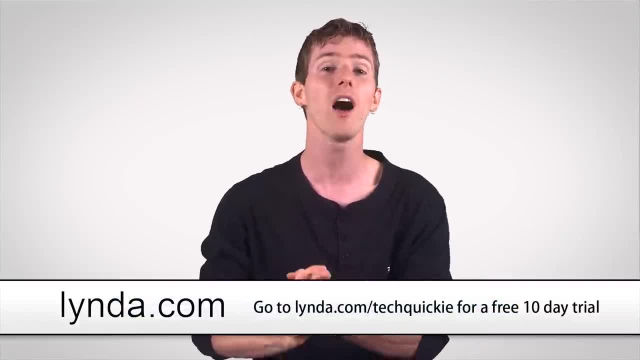 This is what happens when I don't have notes. Your Lyndacom membership gives you unlimited access to all of these topics, all for a flat rate starting at just $25 per month. So whether you're looking to become an expert, you know, brush up on a hobby. 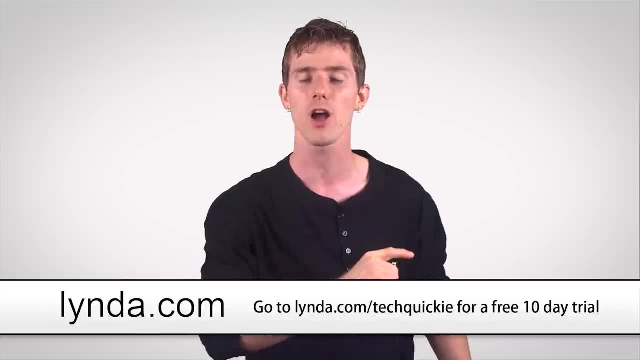 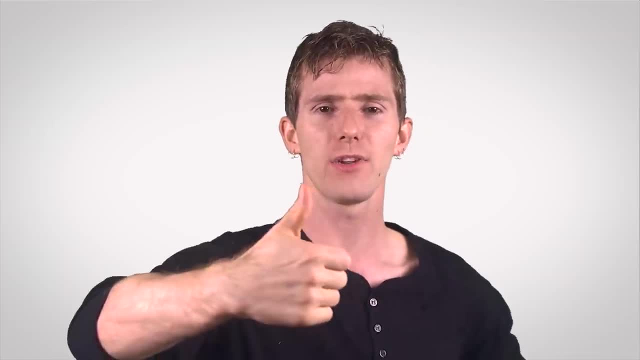 or whatever. if you just like learning, then you can visit Lyndacom slash Techquickie to get a 10-day free trial. So thank you guys for watching. Like this video if you liked it. Dislike it if you thought it sucked.